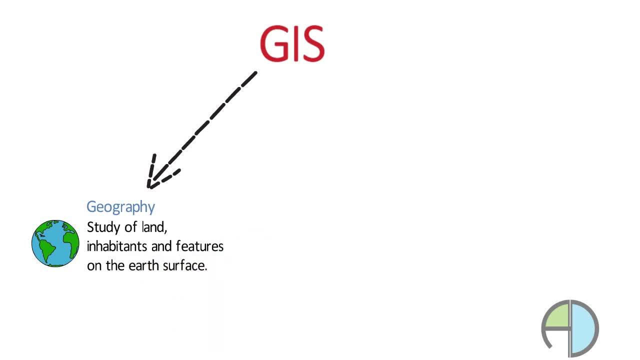 I stands for information. Information talks about details of the features on the surface of the earth. For example, name of a building is an information. S stands for system. System is technology and methods that are used to capture objects on the earth. System is technology and methods that are used to capture objects on the earth. 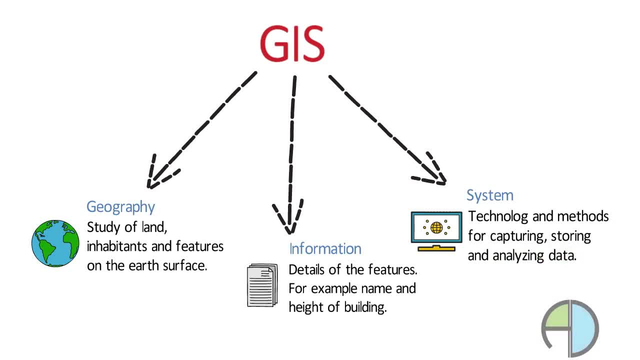 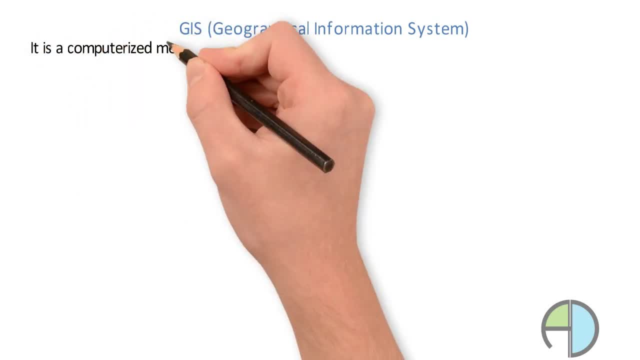 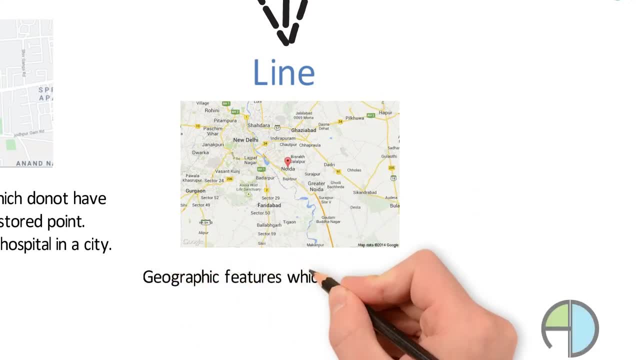 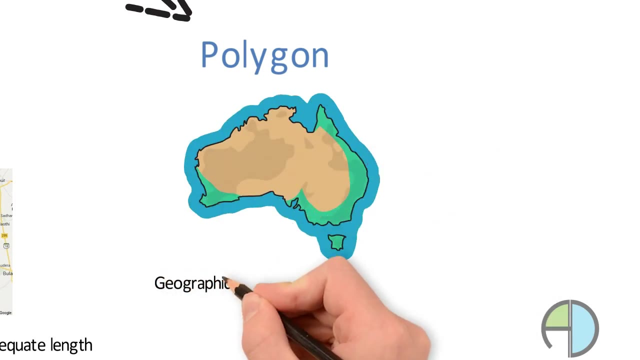 There are two data types involved in GIS system: spatial data and unknown spatial data. Let us understand spatial data in more detail. Let us understand spatial data in more detail. There are also different Tasks involved in GIS…. There are two Tasks involved in GIS system: spatial data and unknown spatial data. Let us understand spatial data in more detail. 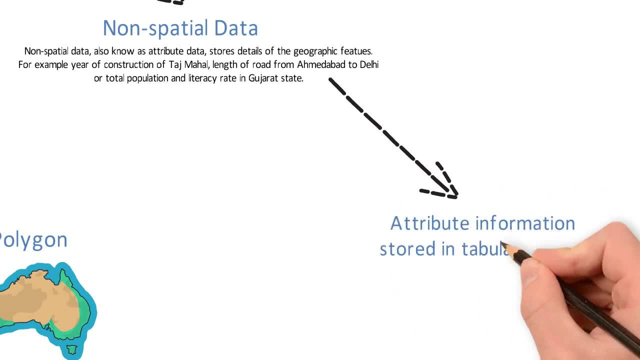 There are two information. it is mostly stored in a tabular format in the database. there are various data types that are supported. for example, name of the building is stored as a text, height of the building will be stored as a numeric, and then construction date will be stored in date boolean. 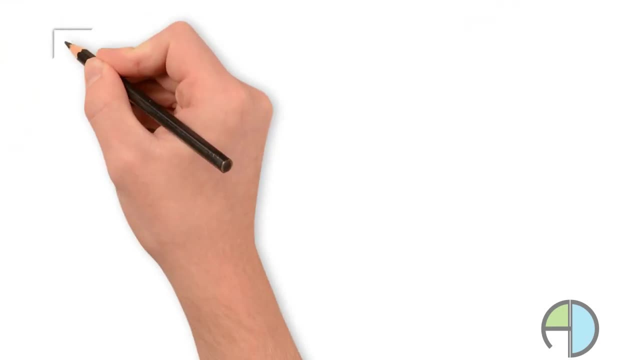 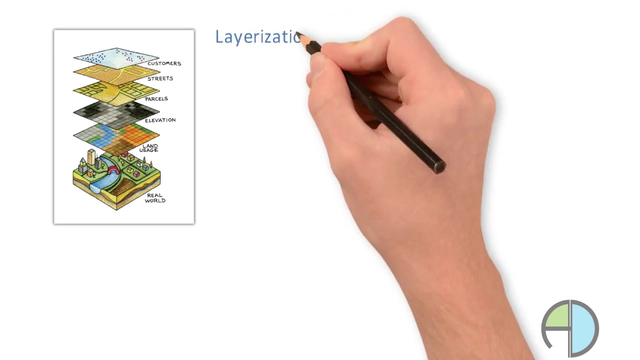 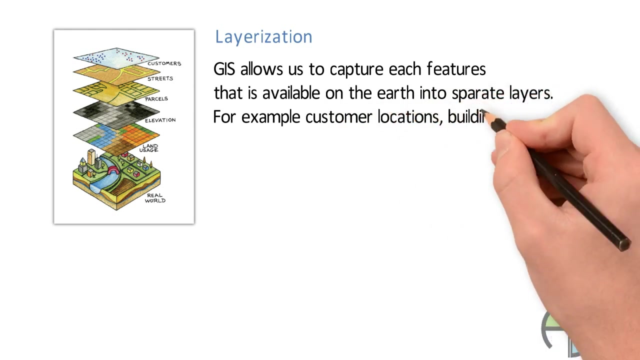 is also one type of data type. the basic building block of a gs system is layer. layer is nothing but logical grouping of similar objects. so gs system allow us to capture each feature that is available on the earth into separate layers. for example, customers can be combined into a. 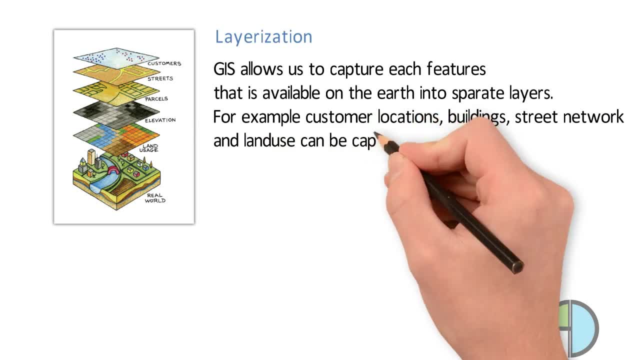 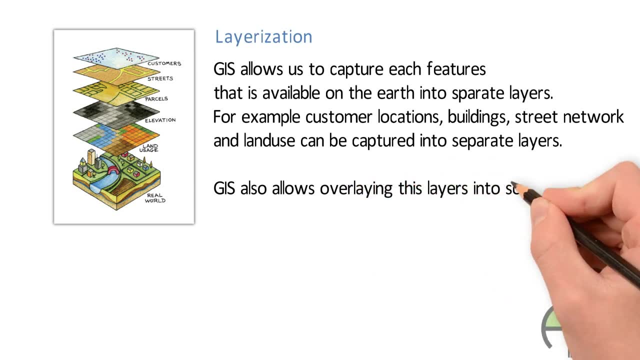 separate layers. same way, buildings, streets and land use can be captured into separate layers. ultimately, gs system will allow us to display all these layer on top of each other, and we can also display all the layers on top of each other. and we can also display all the layers on top of each other, and we can also display all the layers on top of each other. 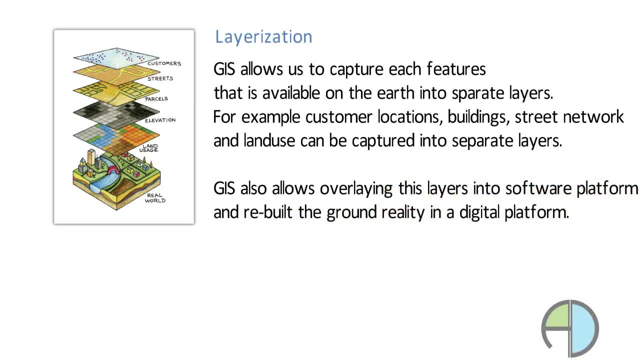 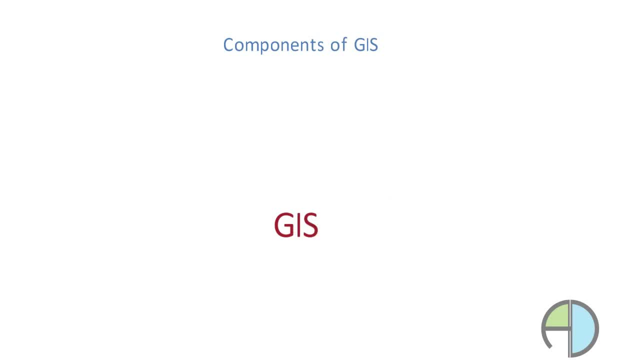 And then we will be able to rebuild the ground reality in digital platform. Let us talk about components of GIS. Basically, there are five components of GIS. First component is a hardware, That is, the server and computers that we use for running the GIS application.